substance per day. What's interesting is that the generator is a non-compact solar panel. This is the only way to make a supervisor use this solar panel. The generator has a solar panel that can complete energy and heat the land. The generator is a show-and-vollence system. When required, the ini is the first. 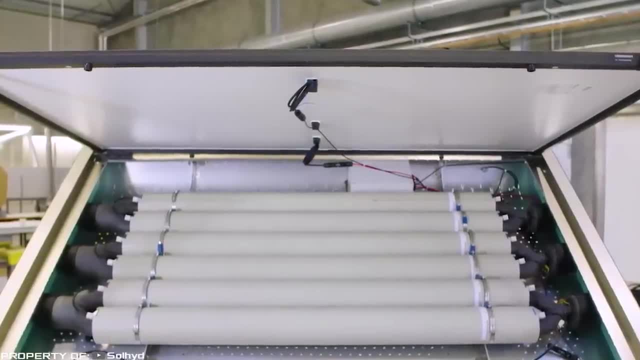 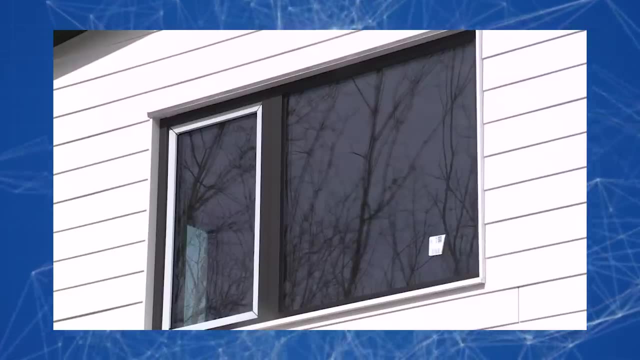 to use the solar panel. If the generator is used, you must turn off the solar panel before charging it. The conversion efficiency of such a panel is 15%, which is currently a world record In terms of practical application of this technology, according to researchers' opinions. 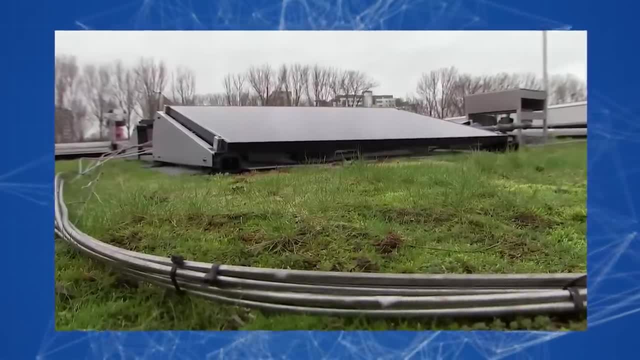 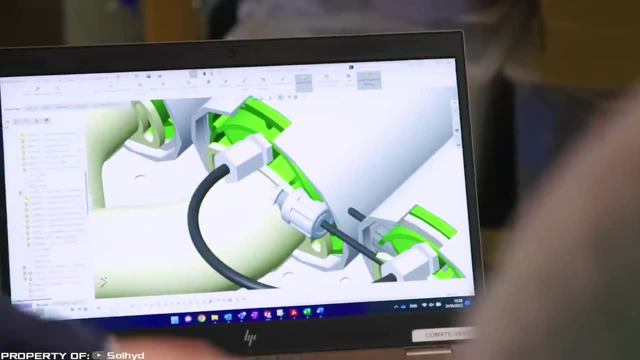 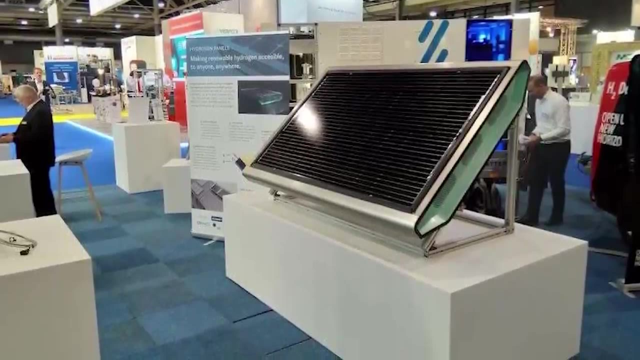 you can easily get through the winter with 20 of these panels on your roof. The only requirement is that your home should be well insulated. The panels are not yet ready for large-scale production, but the possibility of small-scale manufacturing is already being considered. 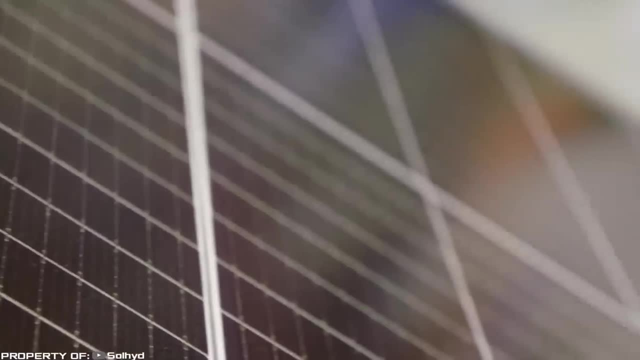 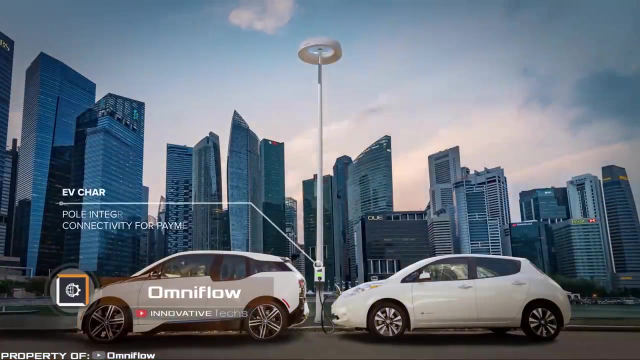 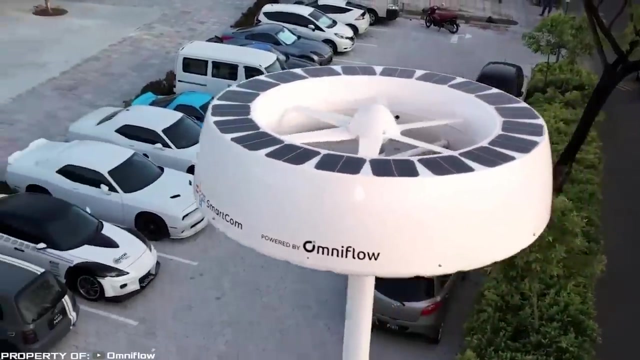 Therefore, it is quite likely that the hydrogen platform may appear on the market as early as 2030.. OmniFlow combines the properties of two previous inventions: wind turbines and solar panels. Thus, the equipment can accumulate and convert not only wind energy but also solar energy. 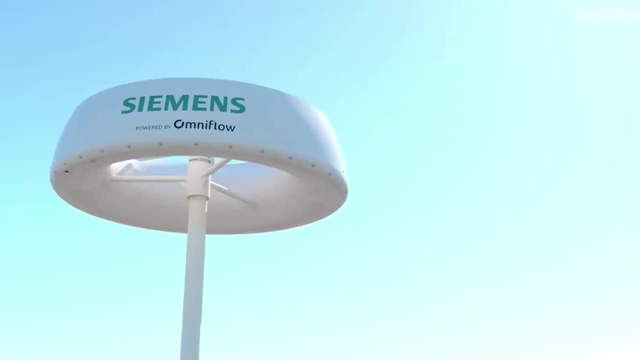 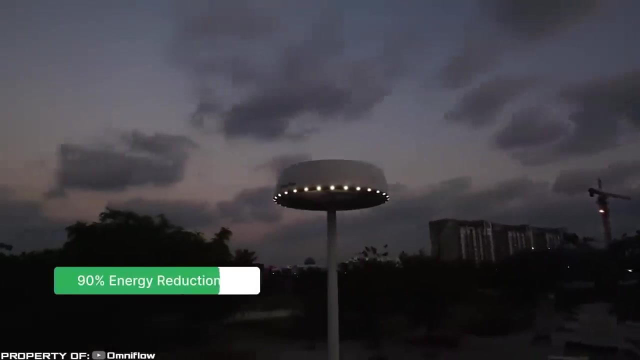 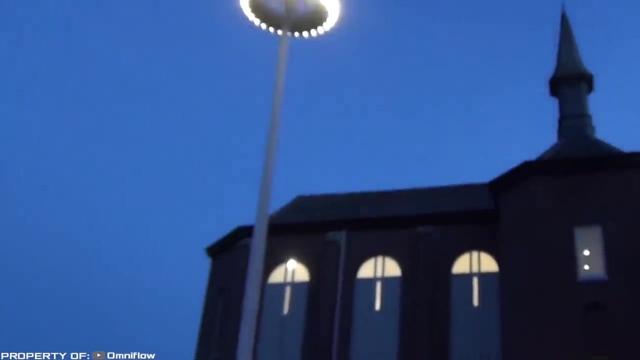 Unlike other similar devices, the generator is positioned parallel to the ground. This is due to the special design of the turbine, which operates on the principle of an airplane wing. Moreover, the device can work regardless of the wind direction. The maximum power of the wind turbine is 3000 watts. 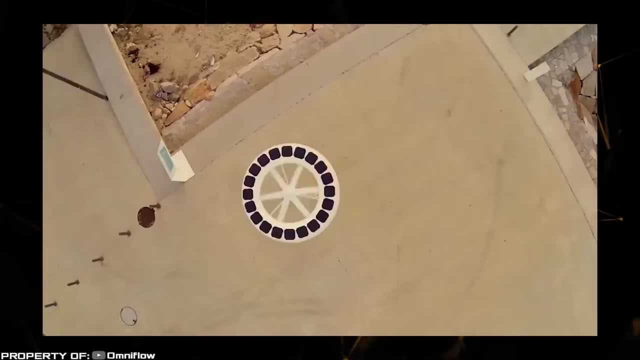 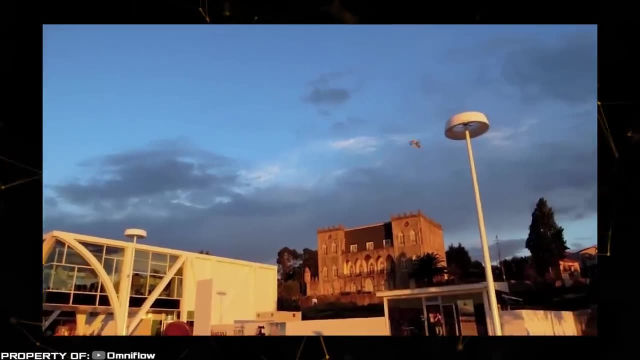 The device's blades start rotating even at a wind speed of only 1.5 meters per second, which is likened to a gentle breeze that can barely be felt on the face. It is anticipated that such equipment will serve as an excellent replacement for regular street lights. 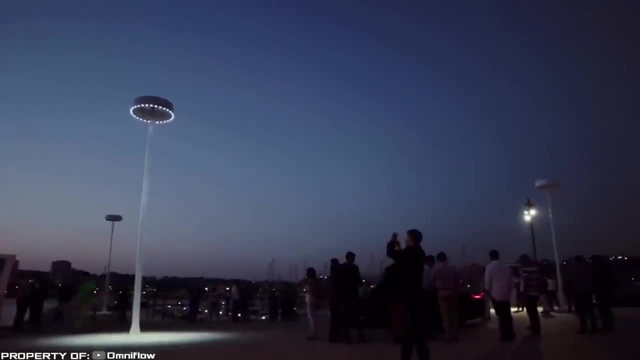 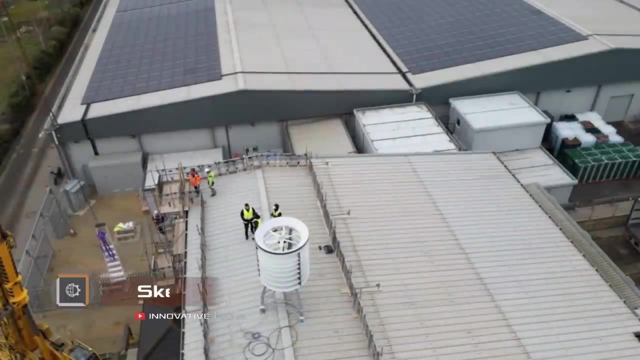 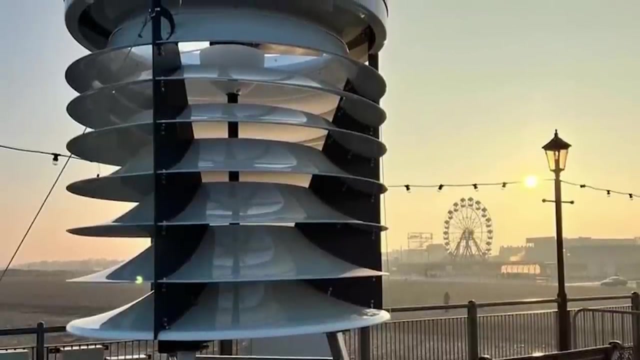 Currently, several test samples of these hybrid installations have already been installed in the harbor of the Portuguese town of Porto. Another option for an unusual wind generator is the Skegnes device. This turbine stands at a height of 6 feet and is installed in a vertical position. 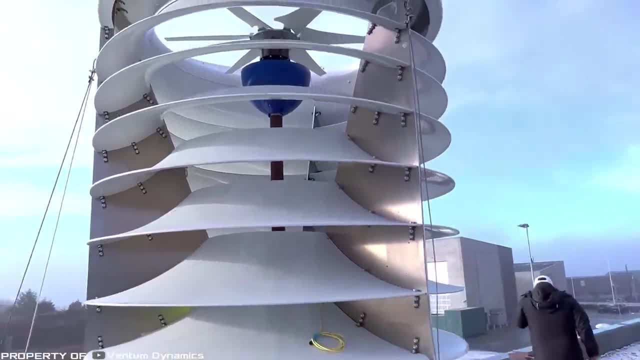 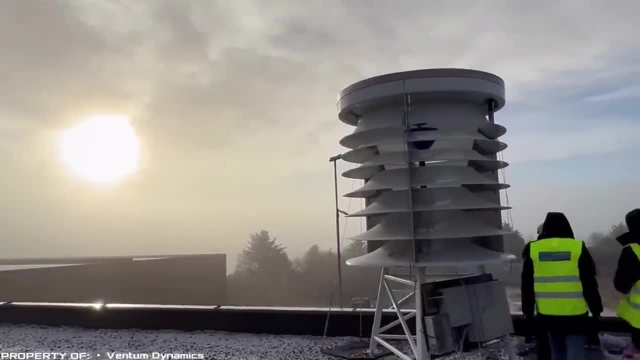 According to the manufacturer, the turbine is designed to be installed in a vertical position. According to the manufacturer, the turbine is designed to be installed in a vertical position. However, this technology will revolutionize green energy. The turbines are omnidirectional, allowing them to capture wind from all directions without needing to rotate, and making them low-maintenance. 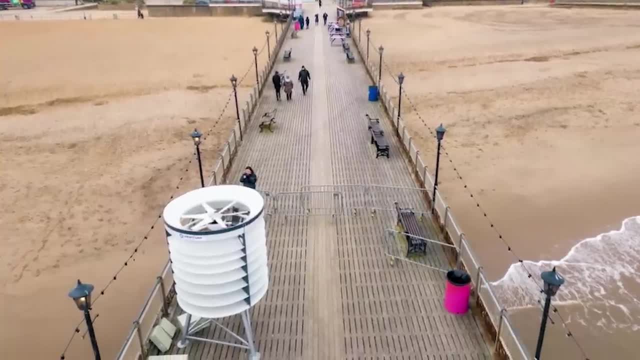 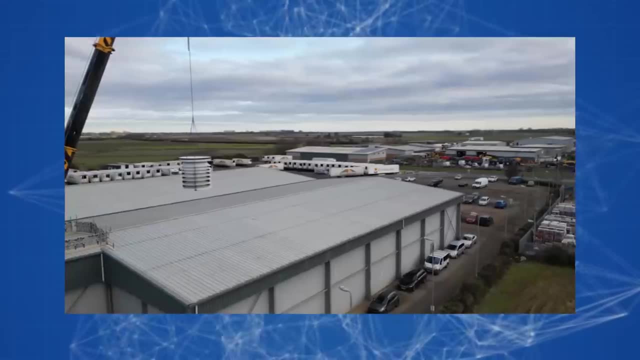 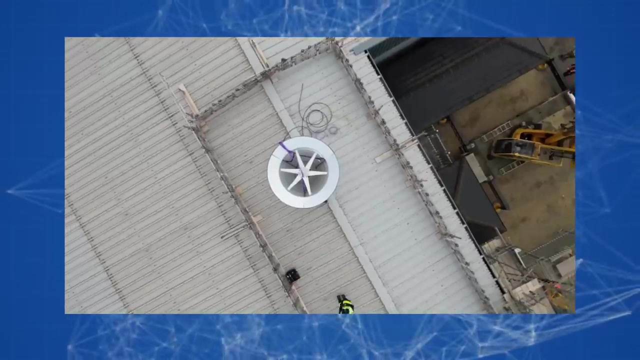 However, this technology will revolutionize green energy. The wind generator can be easily lifted onto a roof using a standard crane. Its silent operation and absence of vibrations make it inconspicuous for people inside the building. Additionally, the generator can be connected to a home's alarm. 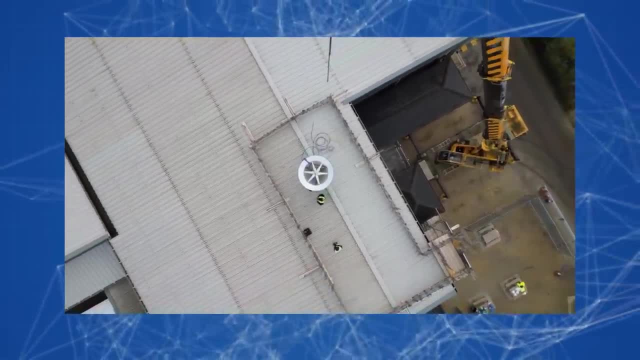 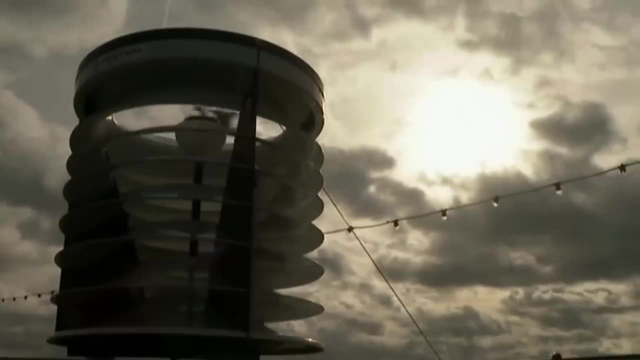 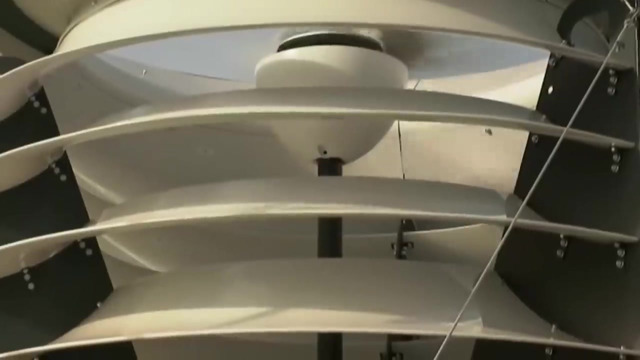 a home's electrical grid as an additional or backup power source. Currently, this technology is in the testing phase. One of the turbines is located on the Skegnes pier and provides nighttime illumination for a historical landmark. The second turbine is installed on the roof of a 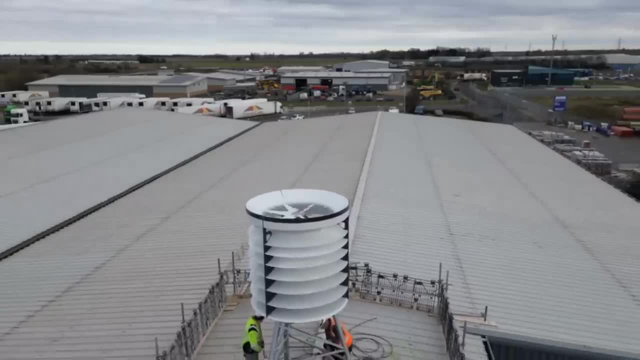 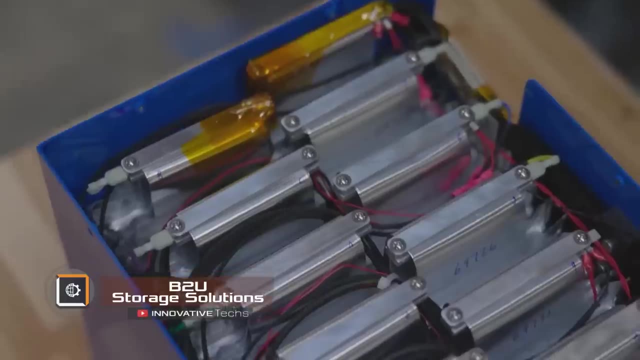 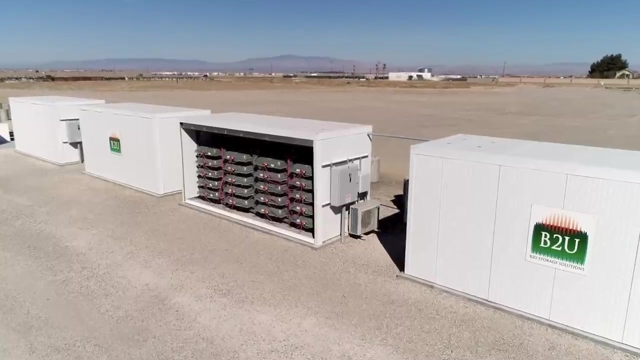 factory in Spalding, providing lighting for one of the factory sections. Over time, the power of an electric car's batteries becomes insufficient to propel the vehicle and expensive disposal becomes necessary. For this reason, B2U Storage Solutions, a startup, has found a new purpose for 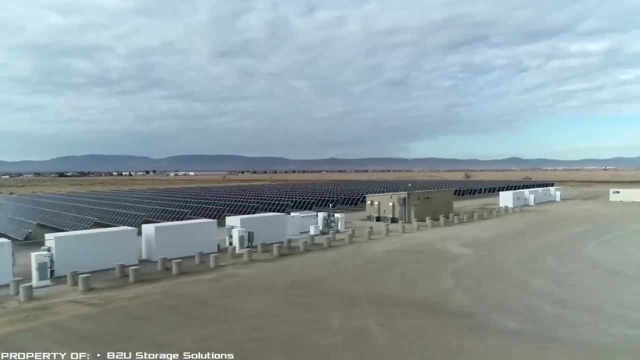 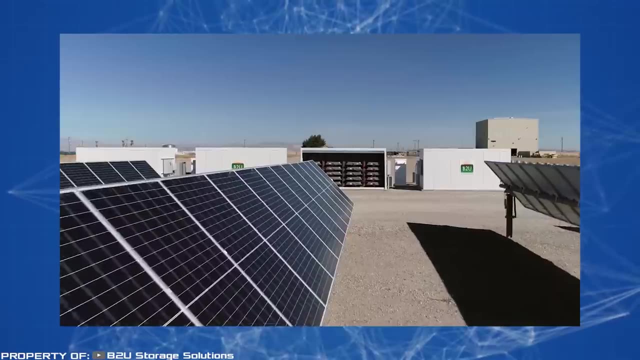 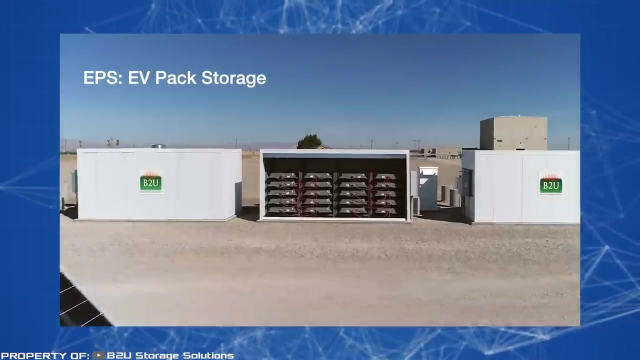 these batteries- Now the batteries that were once installed in electric vehicles with well-known brand names- contribute to California's energy system. Old electric car batteries can be charged up to 85% of their original capacity And used as an additional energy storage system. This significantly reduces the cost of storing. 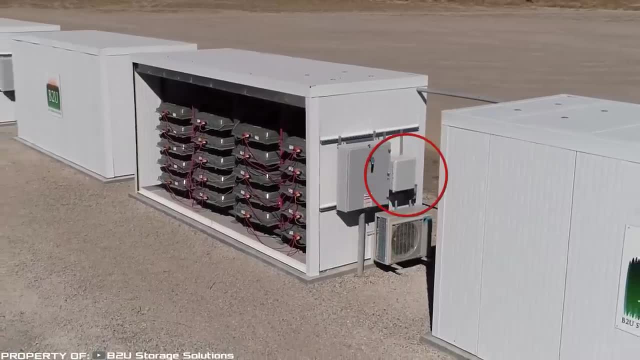 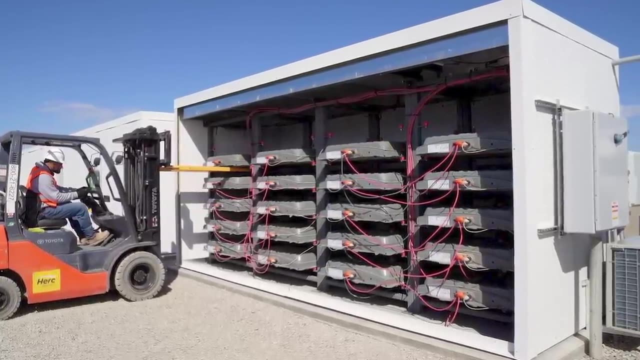 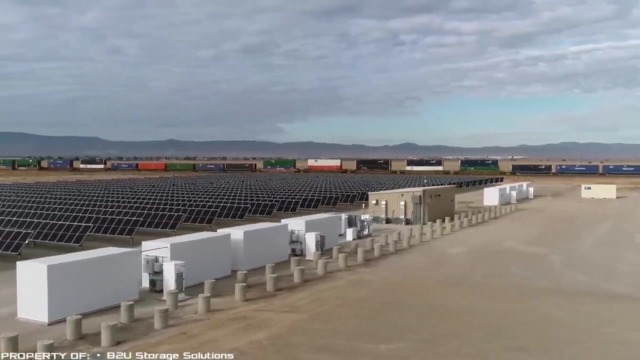 electricity generated from solar and wind stations. According to the company's management, they have access to 1,300 used electric vehicle batteries. All of them are connected to a solar power station located in the city of Lancaster, California, Although the technology is still in. 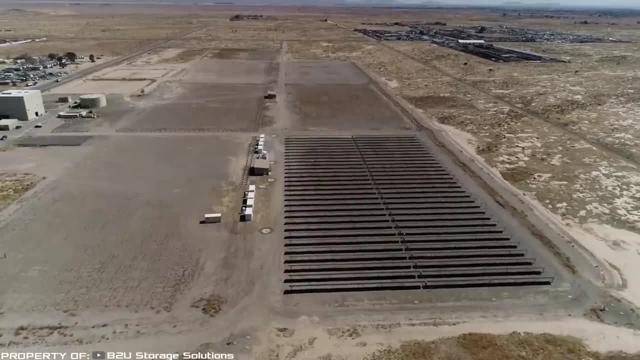 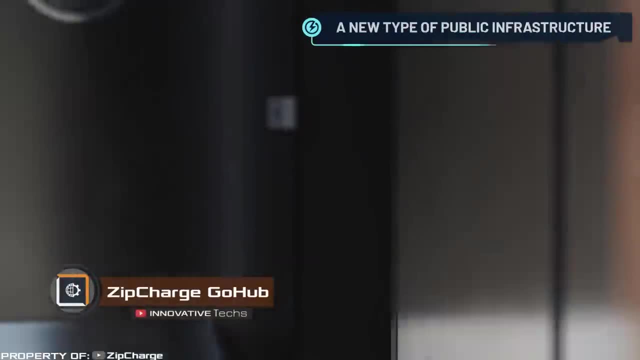 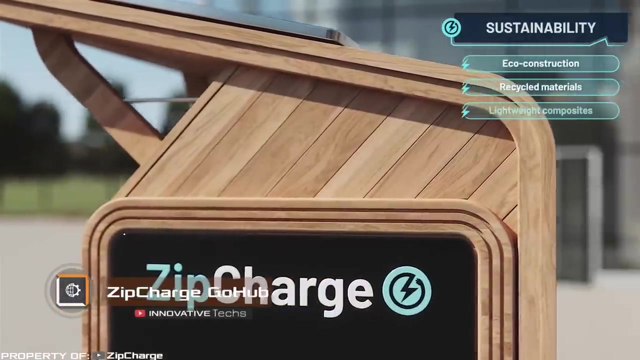 its early stages of development. it has the potential to utilize millions of used batteries in the future. Continuing the topic of electric vehicles, let us tell you about the portable modular charging system for them, Zip Charge Go Hub. The station features a modular design and flexible. 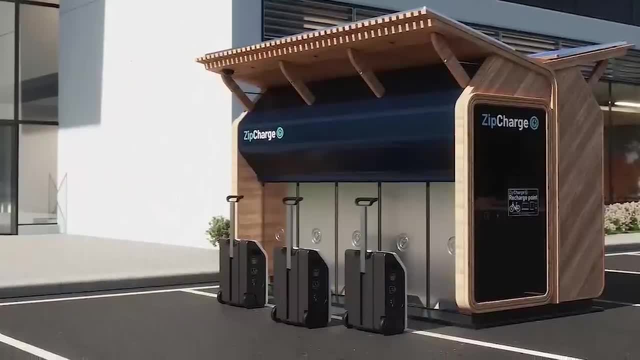 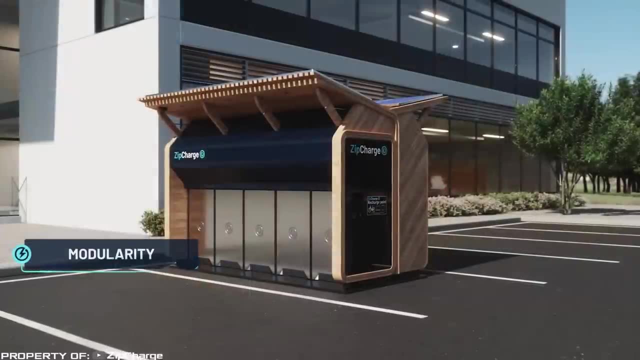 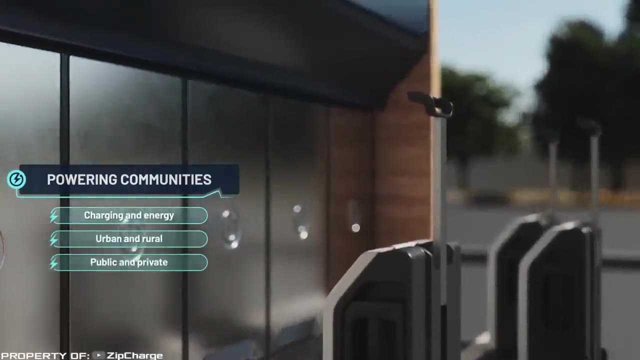 dimension, allowing it to be used in various locations. It can be a parking lot near office buildings or in residential areas. The system is available in two variants, with five or ten portable charging units. Both variants easily fit into a standard parking space. They can also be installed on 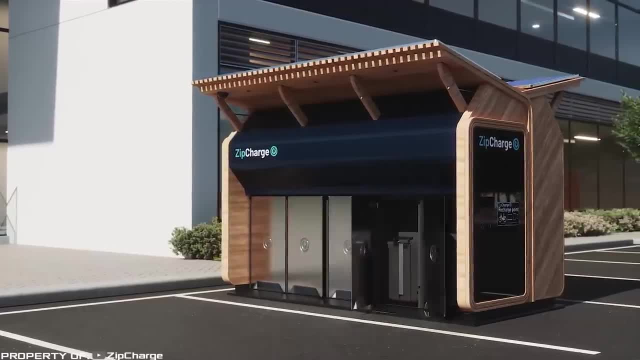 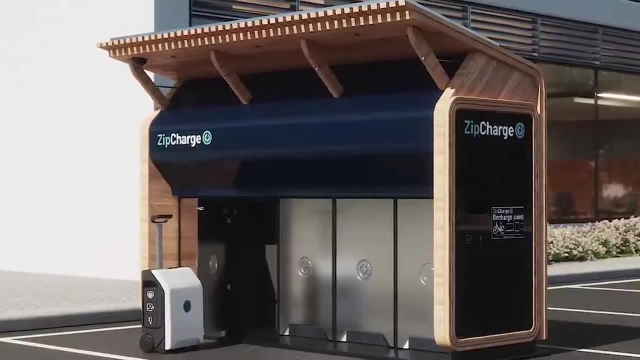 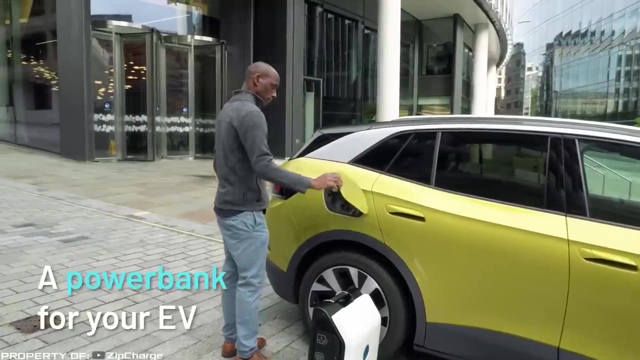 sidewalks or near areas where electricity is already available. Through Go Hub, the charging units will be available for rent 24-7.. When a user approaches the designated compartment, the structure's door automatically opens. The user then retrieves the charging units, brings it to their vehicle and 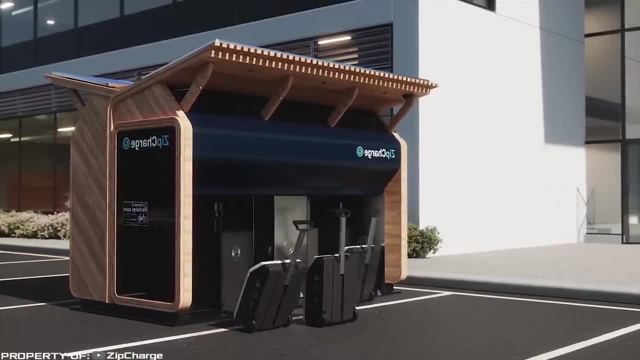 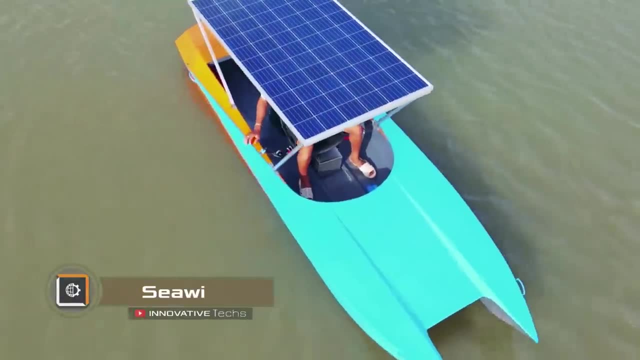 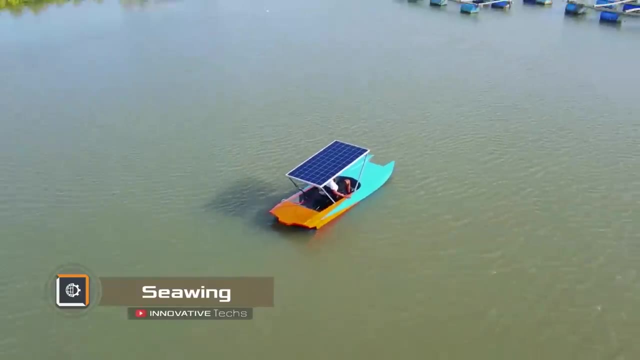 connects it. Once the charging process is complete, the user returns the portable charger back to the compartment. The use of green energy technologies is relevant not only for land transportation, but also for water transport. A shining example of this is the kite called Sea Wing, developed by the French company Air. 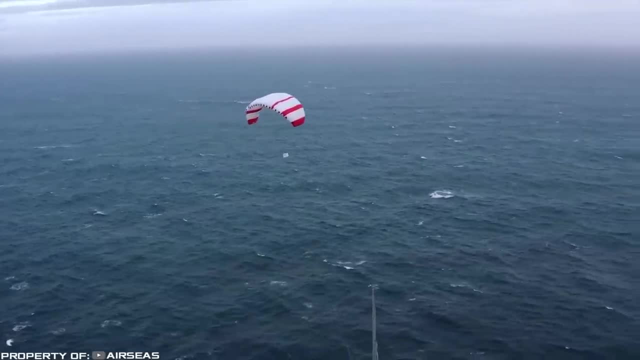 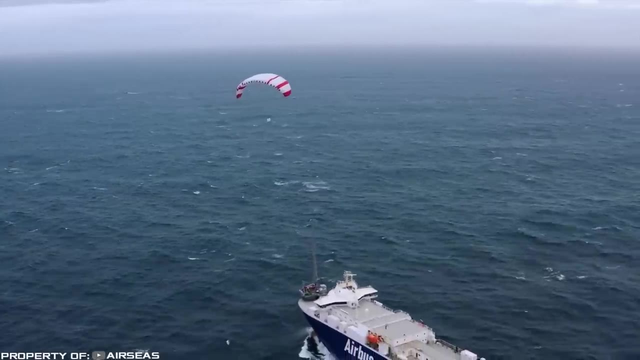 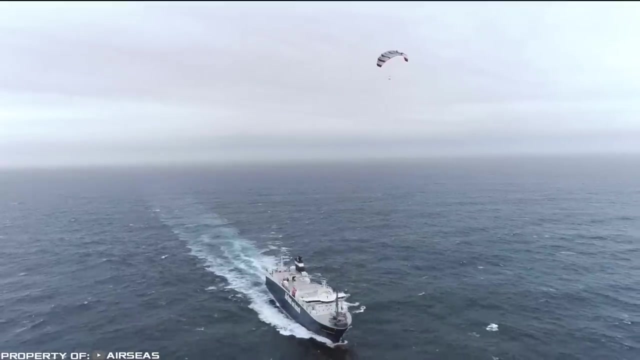 Seas. This airborne kite has a surface area of one thousand six hundred forty feet. Thanks to its large surface area, the kite provides additional thrust, reducing the load on the ship's main engine. According to the developers, this airborne kite can reduce fuel consumption and carbon emissions by 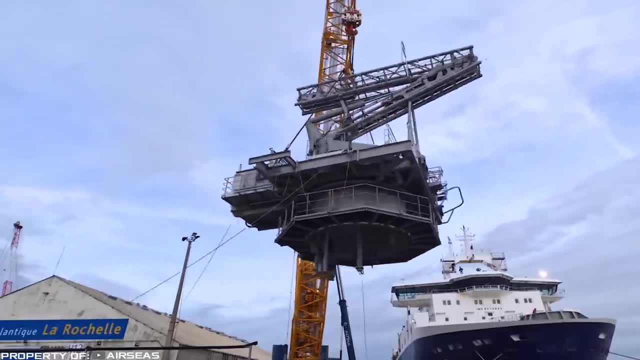 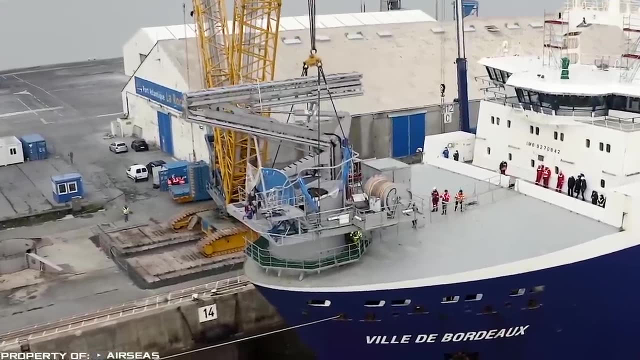 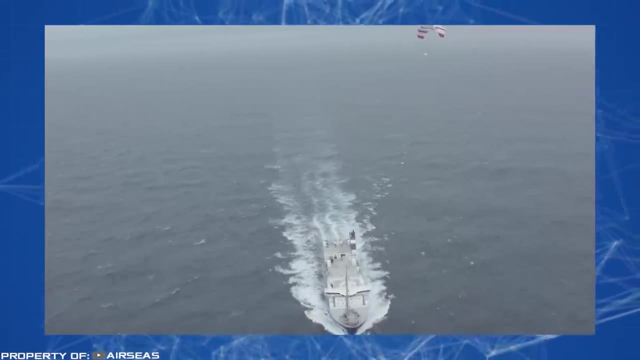 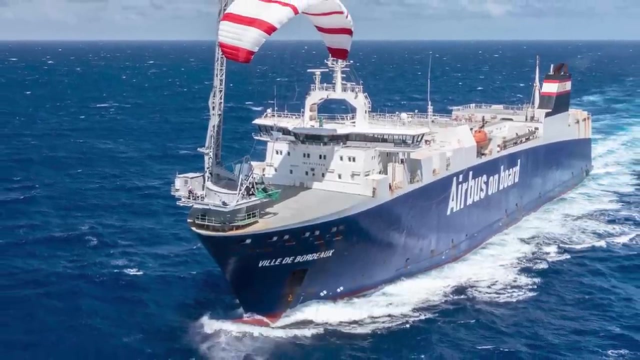 twenty percent. The company also claims that its sail technology can be easily installed on any vessel, with the process taking only a few days. The invention is already being successfully tested on the cargo ship Via de Bordel, which delivers a number of aircraft components across the Atlantic Ocean. This system represents the first step before implementing. 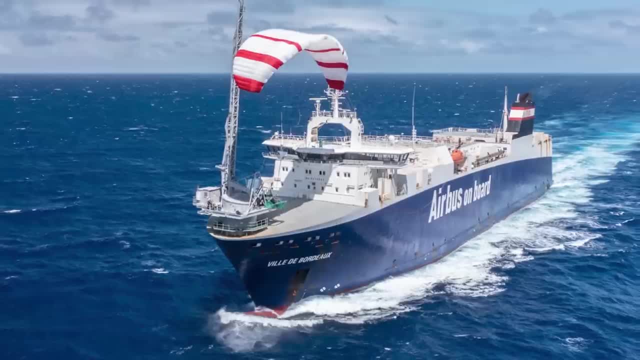 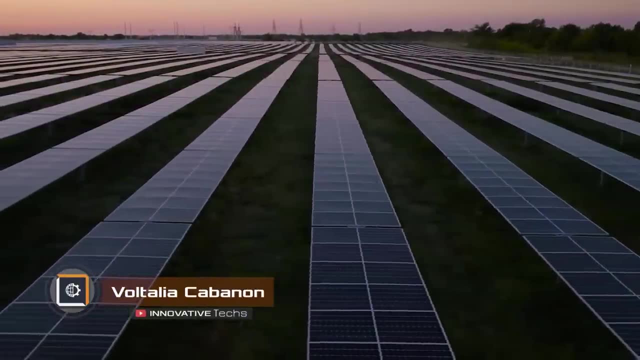 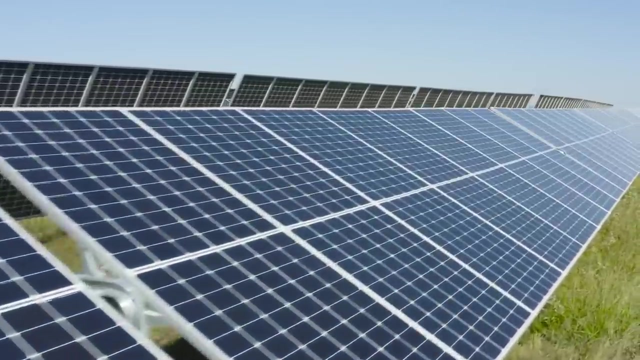 the full-scale serial version of the kite, which will have a surface area of three thousand two hundred eighty feet. Finding areas for solar panel installation is becoming increasingly challenging. Moreover, such structures often occupy fertile land. An innovative solution to these problems comes from research that has been conducted in the United States and the United States. 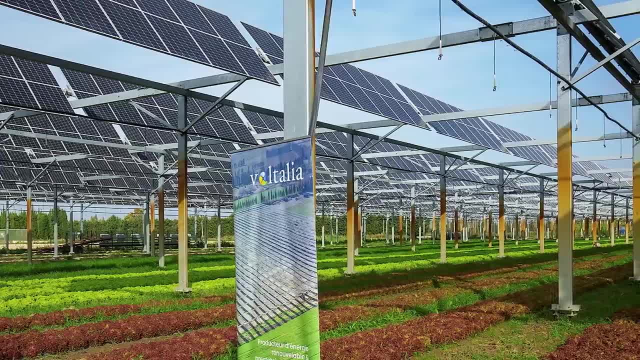 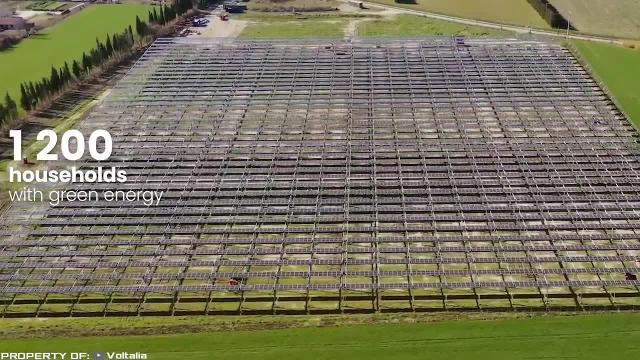 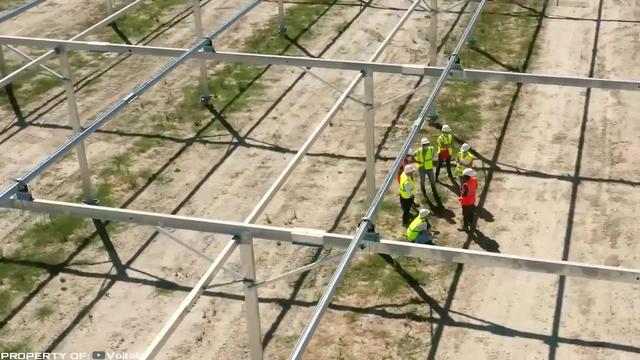 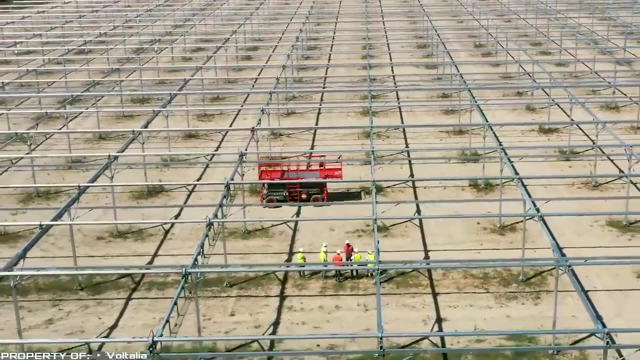 An innovative solution to these problems comes from research that has been conducted in the United States and the United States. An innovative solution to these problems comes from research that has been conducted in the United States and the United States REPS. At the beginning of February, HEядCS identified an area of three hundred twenty-five cubic meters that would cover a quarter of the American. atmosphere. The 6hehe fish servir apartment property of the captain aircraft. Magical Hawler's camera option features are: aiczal 나도. back to Mrs Goldberg and nuestra la gente intac 막light video. we wanted to focus a little bit more on the potential stability of Mars. 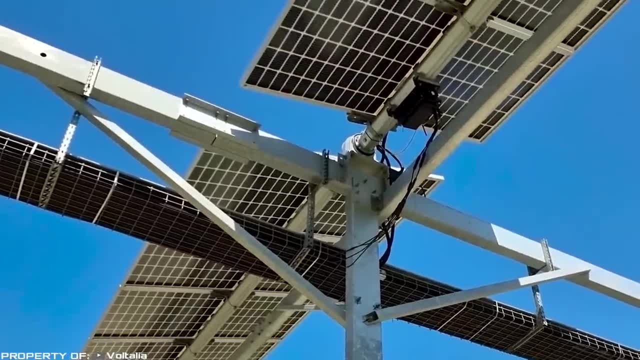 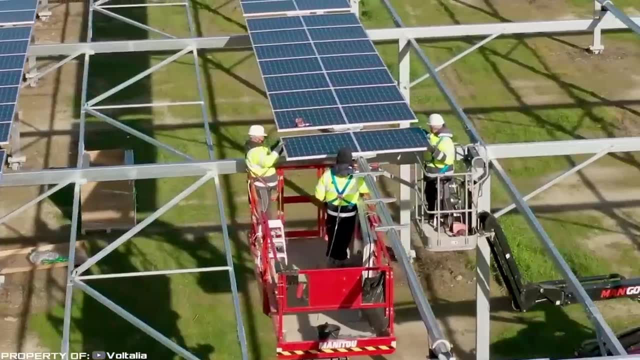 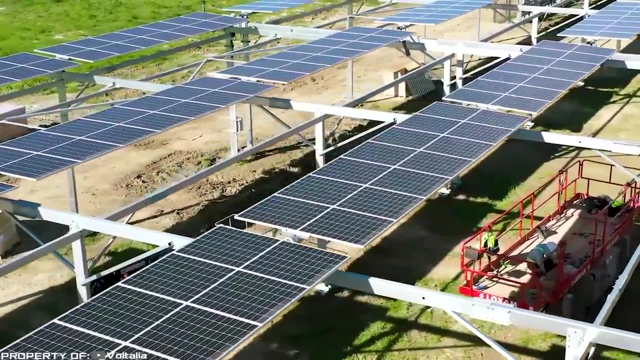 process. The station also has the capacity to generate up to 3 megawatts of power, which is sufficient to meet the electricity needs of over 4,000 people. The entire complex occupies an area of 4.5 hectares and the project implementation cost.